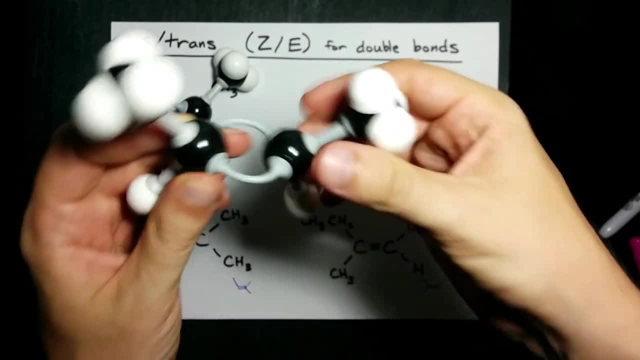 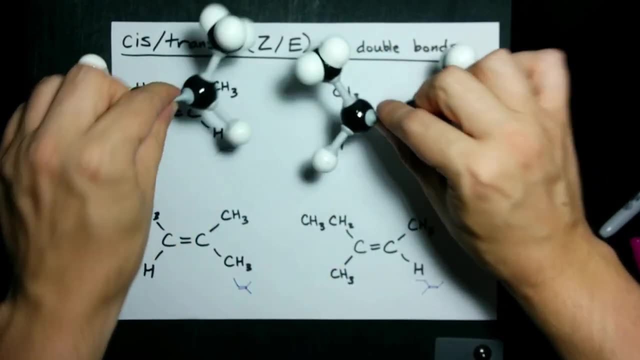 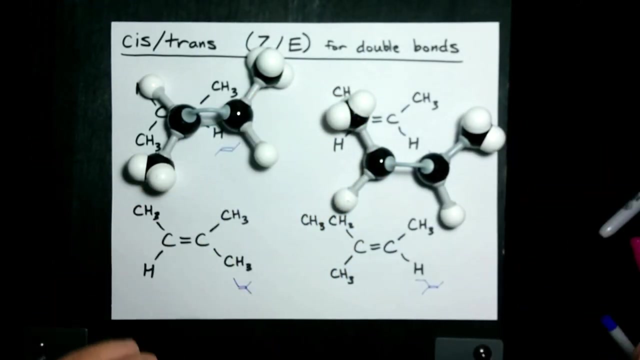 and they have a double bond at carbon number 2.. But because double bonds can't rotate the same way that single bonds can, it means that these two- one where the CH3 groups are across from each other and one where the CH3 groups are on the same side of the plane of the double bond- 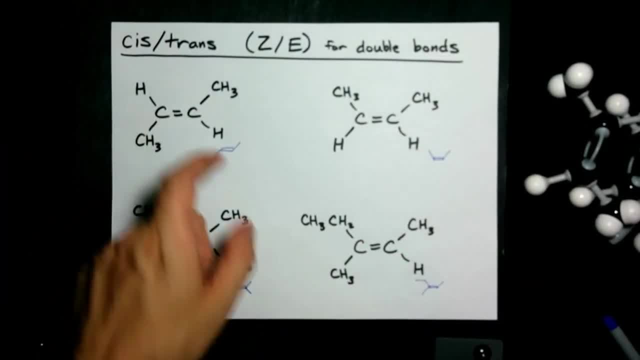 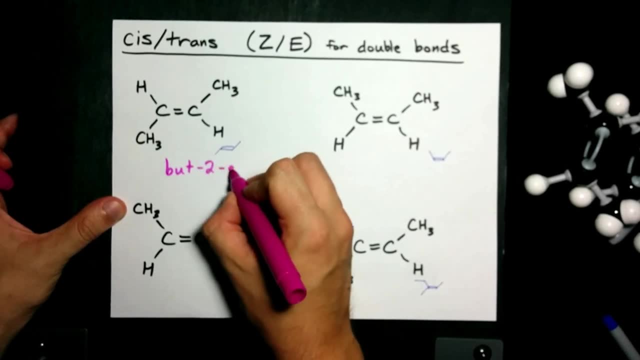 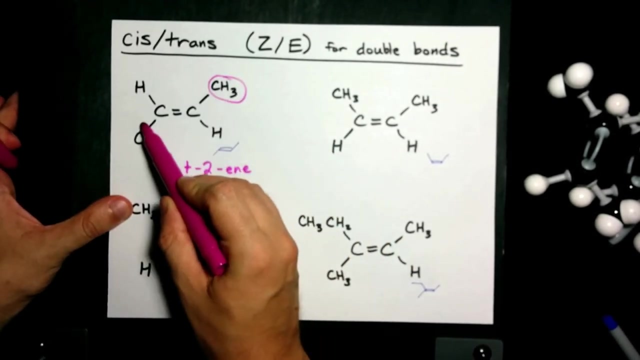 are different. Alright, take a look Here. we have a 4-carbon long chain that makes it bute and a double bond at carbon number 2, which makes it 2-ene. But the CH3 groups are on opposite sides of the plane of the double bond. 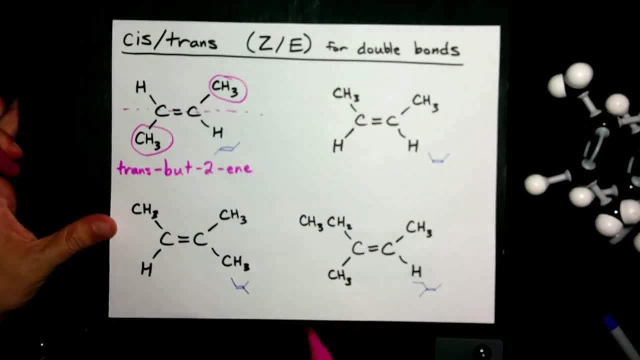 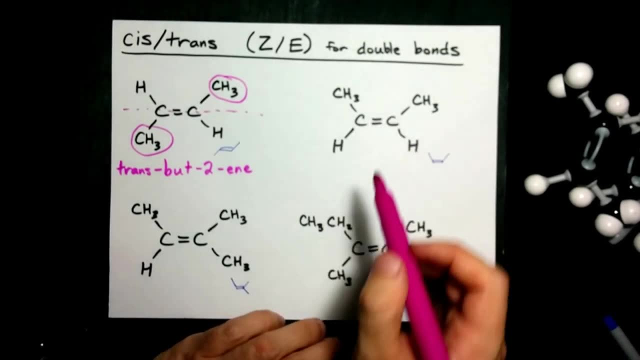 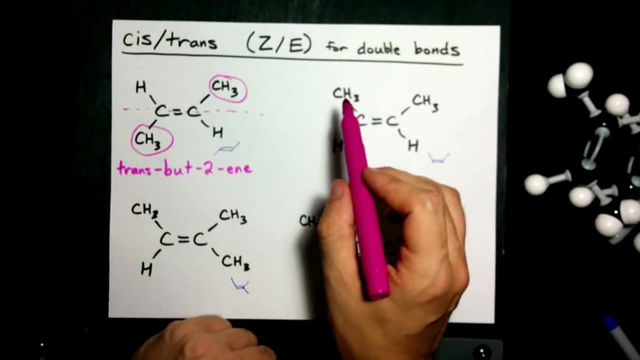 So we preface the name with trans and the official name for this molecule. one of them is trans-butane. Here we have the exact same thing: four carbons in a row with a double bond starting at carbon 2,. 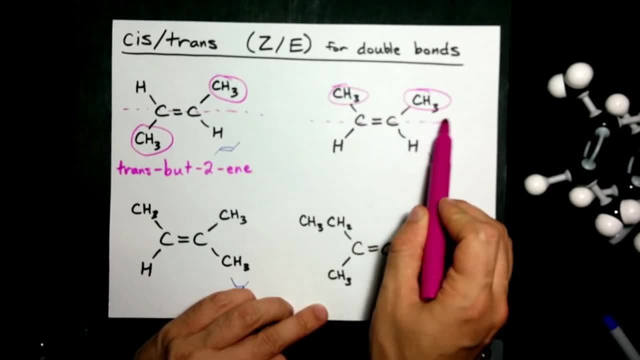 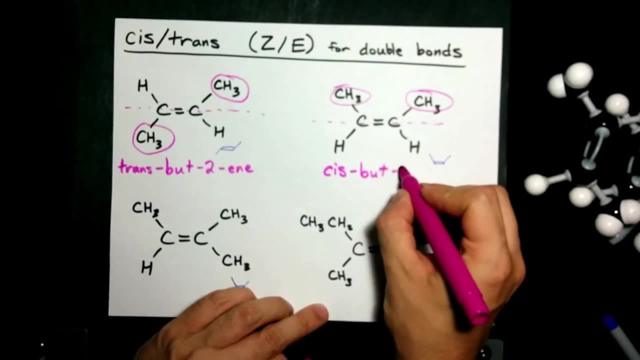 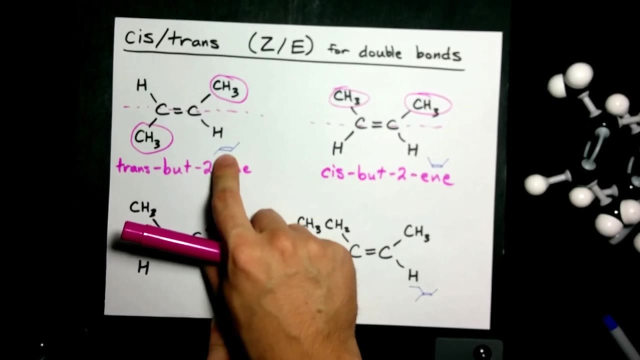 except the CH3 groups are on the same side of the double bond. When they're on the same side, we use the prefix cis. If you're into ball and like if you're into the skeleton models for organic compounds, this molecule is this one. 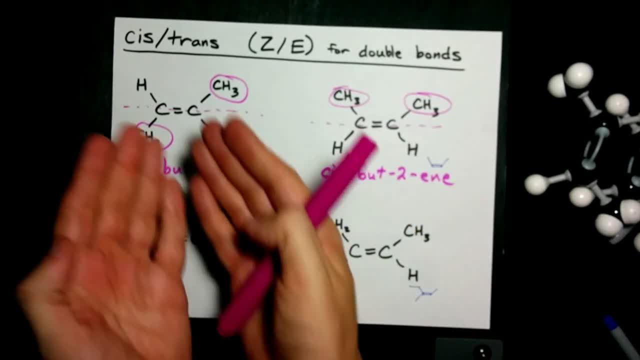 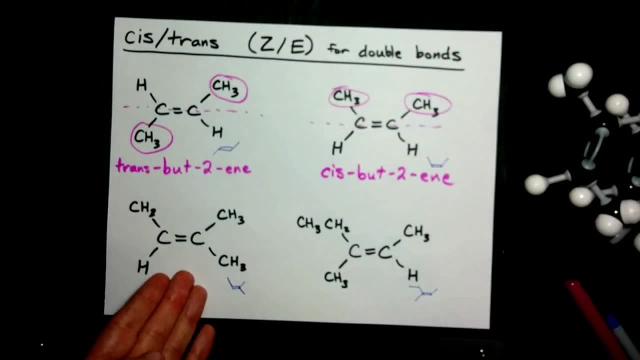 And this molecule is that one. But what I really want to get across is that trans means across, cis means same side. Take a look at this molecule. On this side, or attached to this carbon, we have an H and a CH3.. 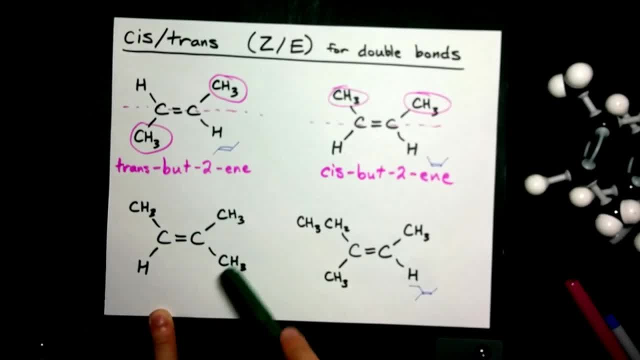 On this carbon, we have two CH3 groups. If we could rotate this double bond, which we can't, if we could, these would replace each other, And it would be like this And it would still be the exact same molecule because they're both CH3s. 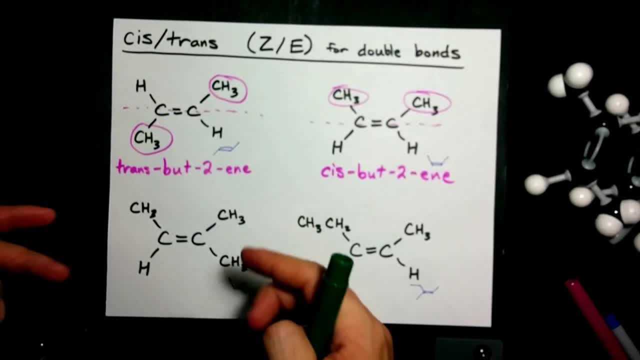 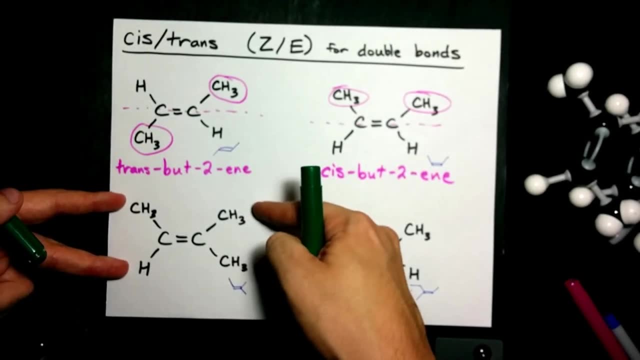 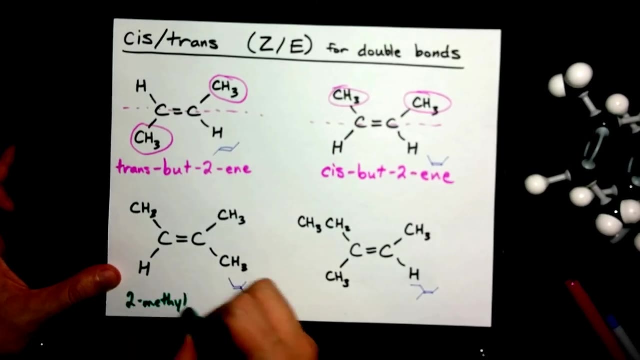 In order to even have cis-trans isomers, you need two different things attached to this carbon and two different things attached to this carbon. Otherwise it's not cis-trans isomerism at all. This is just straight up. 2-methyl-but-2-ene. 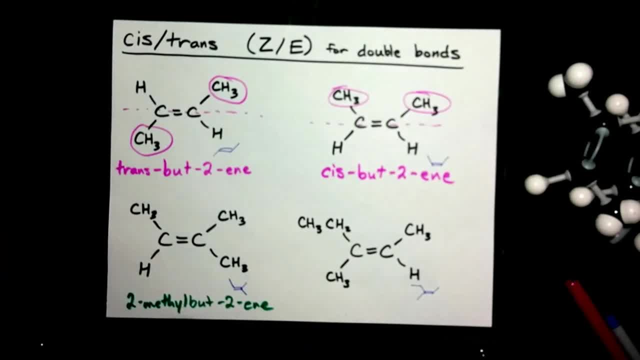 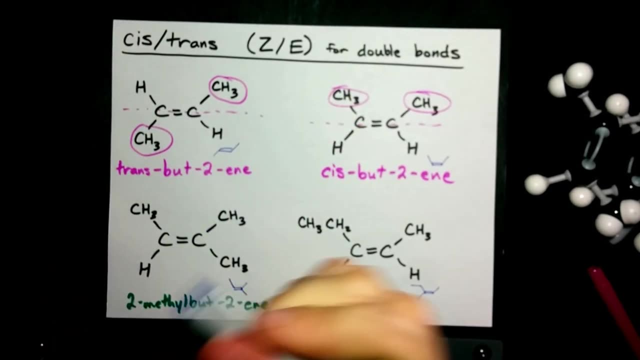 And that's it. No cis-trans to worry about. I just want to also get across what happens if you have a more complicated molecule. You probably just took for granted that I said the CH3 groups were the important ones here. What it really comes down to is a set of rules called Kahn-Ingold Prologue. 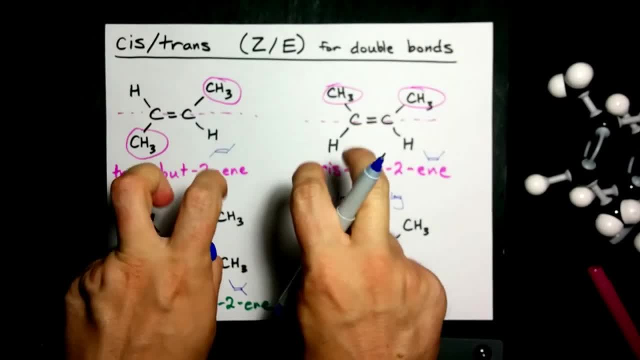 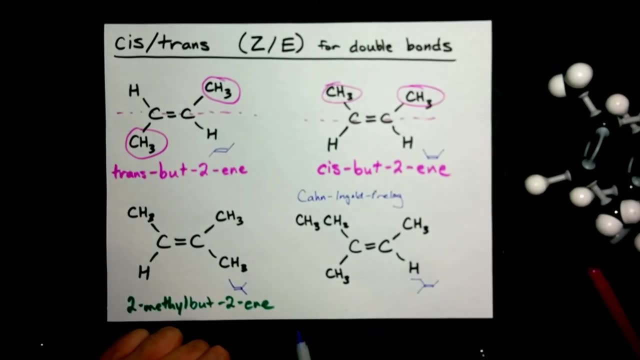 which tell you which groups have precedence over each other, This carbon atom, which has a methyl group and an H attached to it. well, you have two choices, for which one gets precedence. It's attached to an H and a C, and carbon has a higher atomic mass than hydrogen does. 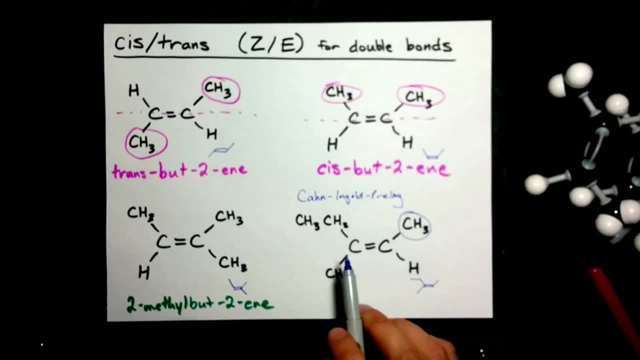 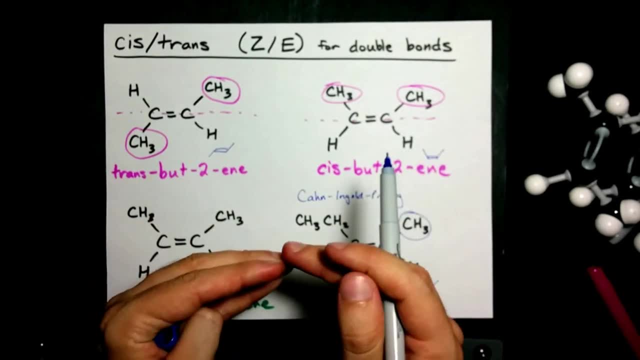 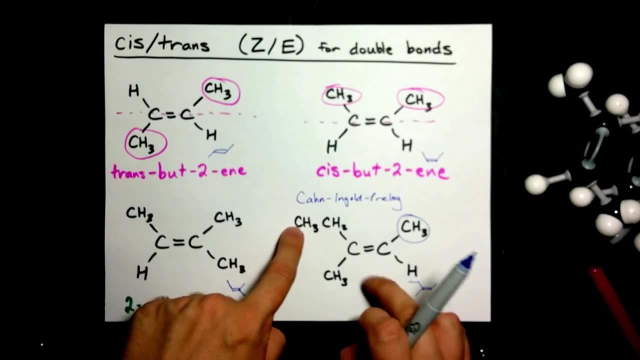 so the methyl group wins out. Taking a look at this carbon, it's attached to a carbon here and a carbon here. Those are the same, so we have to branch out further. This carbon was connected to three hydrogens. This carbon was connected to another carbon and two hydrogens. 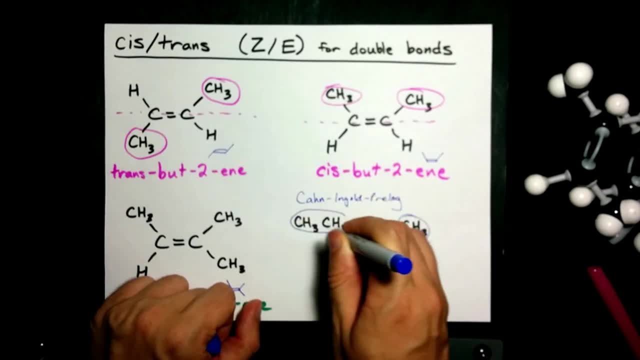 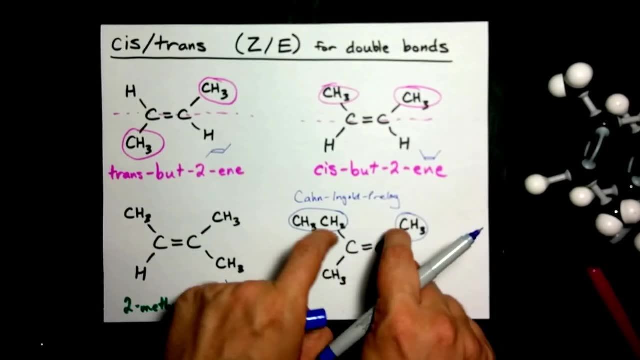 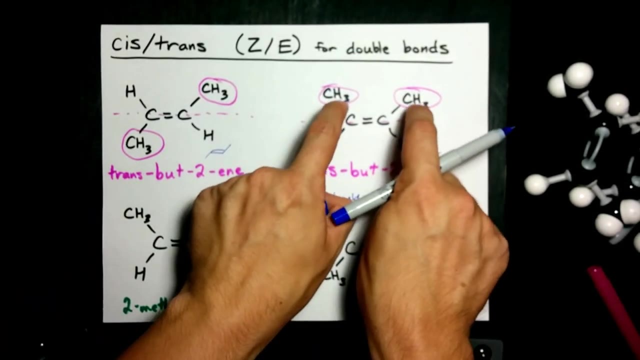 That carbon beats out the hydrogen, so he gets precedence on these two. If you had to do cis-trans isomerism for this, it would be cis, But really cis and trans, I think, are much more for when you have two of the exact same group. 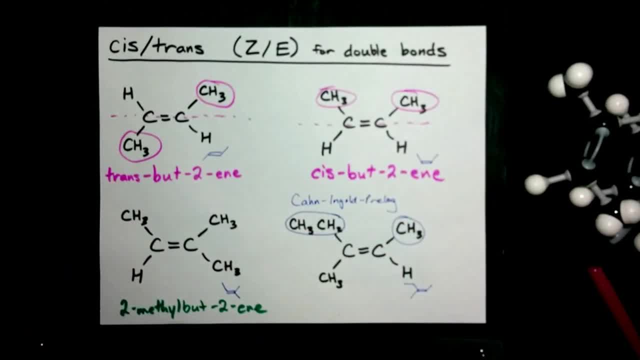 and you're trying to tell people if it's on the same or opposite side of the double bond, The more official or con and gold prologue or IUPAC way of doing this is to say if the two groups that have highest precedence are on the same side. 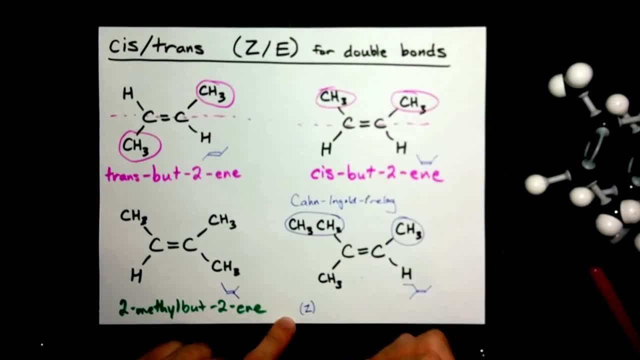 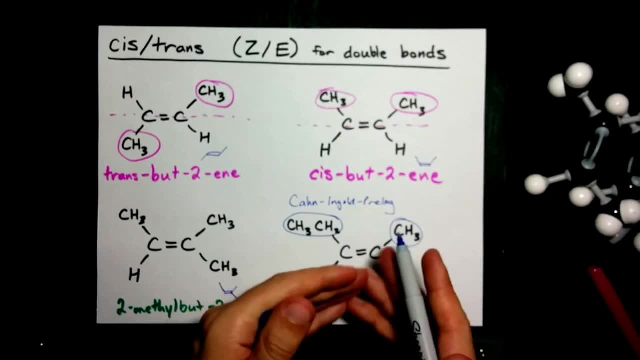 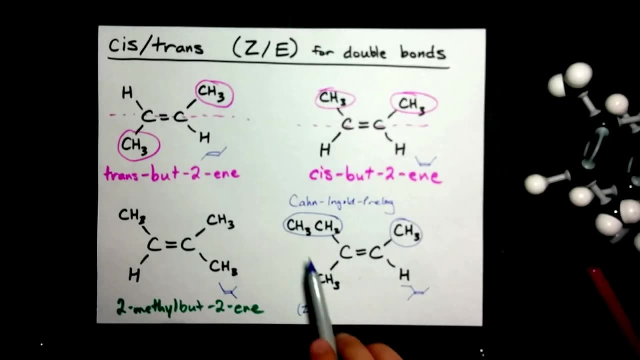 then you preface the name with the letter Z. The Z tells us that the two precedence groups are on the same side, ie they're cis. I'll name this for you while I'm here. It looks like we got a 1,, 2,, 3,, 4, 5 carbon chain with a methyl group sticking off here. 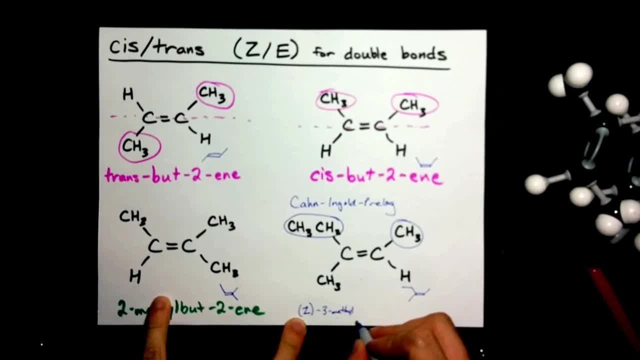 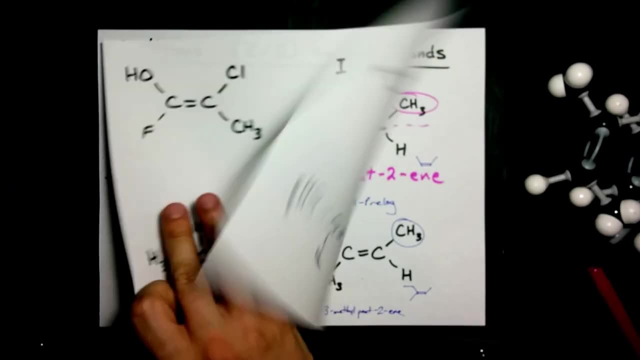 This is 3-methylpent-2-ene, Because there's only one double bond. everyone knows that this Z applies to that too. I created some more examples for you because I know you guys are hungry. Two carbons with a double bond between them. 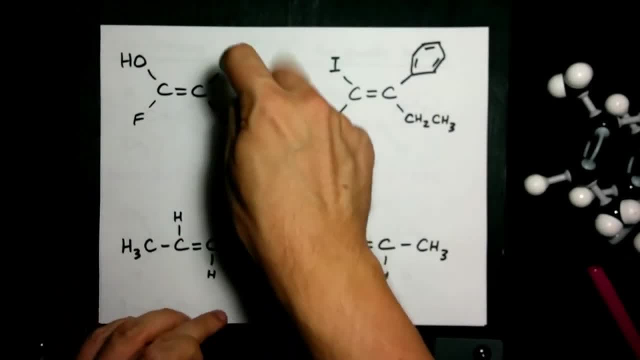 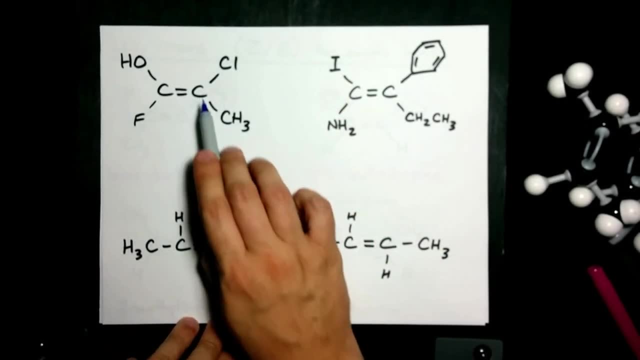 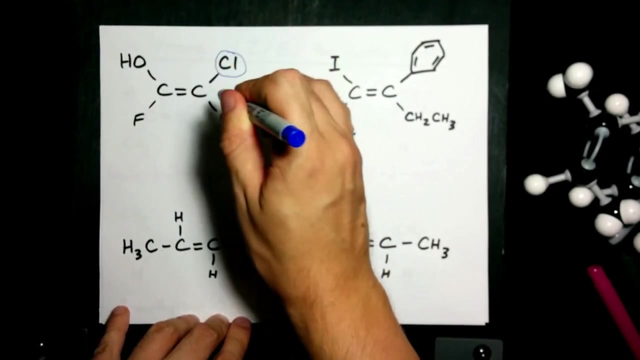 Check for cis-trans isomerism. These are different and these are different. Therefore, we do have it. Which groups get precedence? This carbon is connected to a carbon and a chlorine Carbon weighs 12.. Chlorine weighs 35.. Chlorine wins. 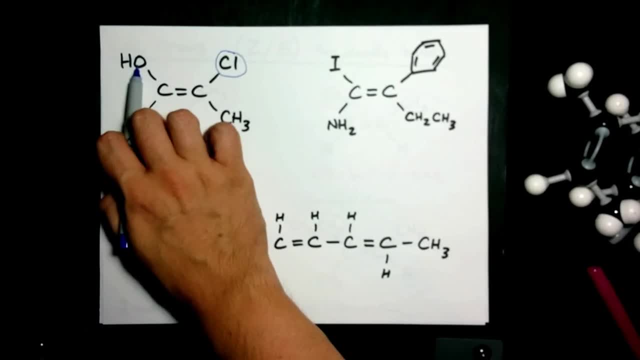 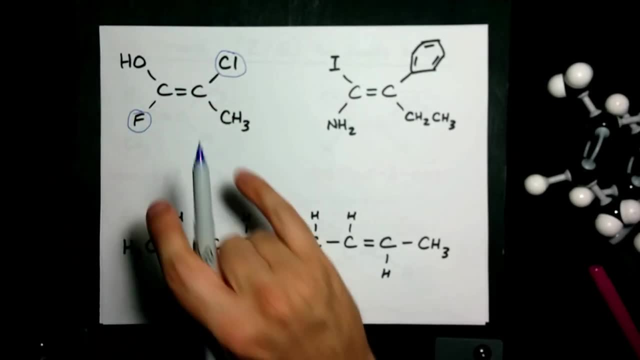 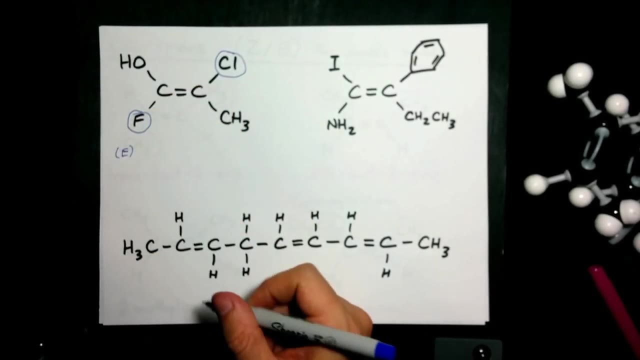 This carbon is connected to an oxygen and a fluorine. That's 16 atomic mass units versus fluorine's 19.. Again, I would hesitate to call that trans, because these two groups aren't even the same thing. I would jump to calling it E. 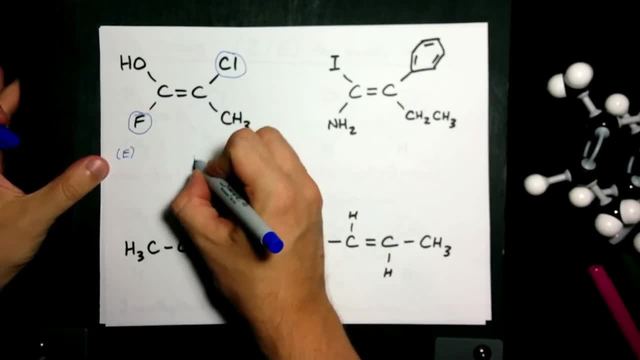 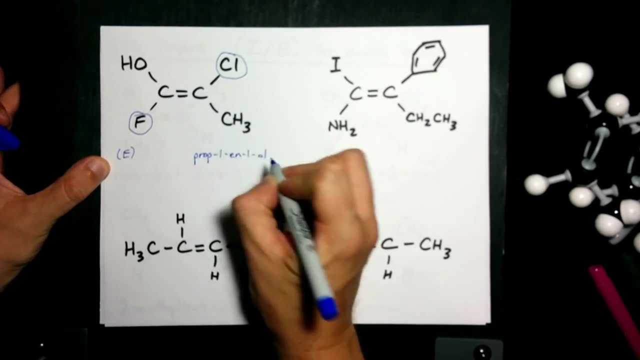 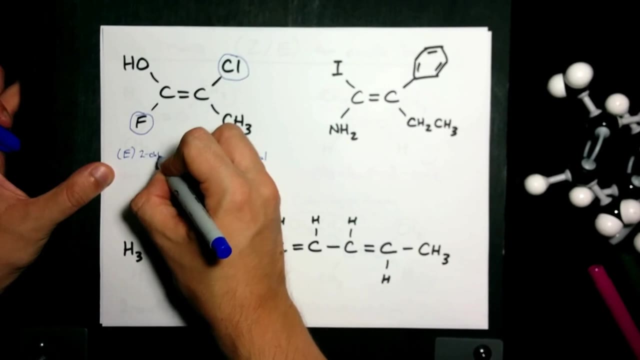 Now I don't particularly want to name this. I'll name it anyways. It's a prop-1-ene-1-ol Because it's an alcohol, But we have 2-chloro-and-ethane. I'm not doing that again. 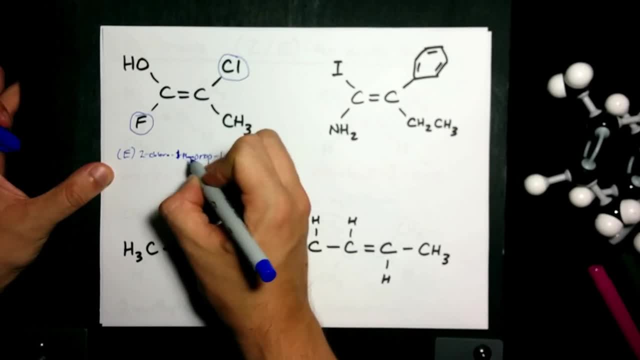 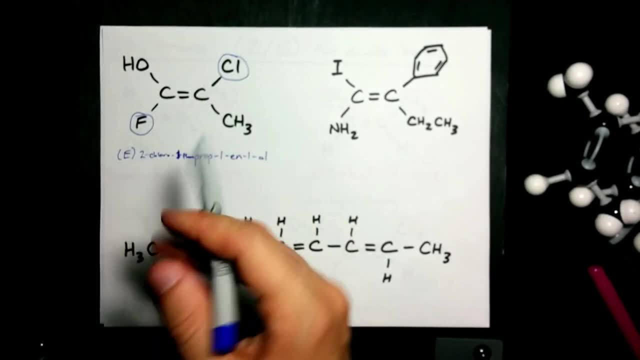 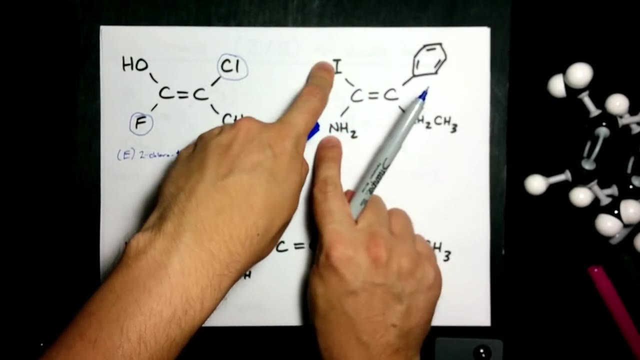 The point is it's E, Because they were on opposite sides, Like trans. Alright, one more. Two carbons with a double bond. I and NH2 are not the same. I weighs 127.. Nitrogen is 14.. Here's a carbon connected to an ethyl and a phenyl. 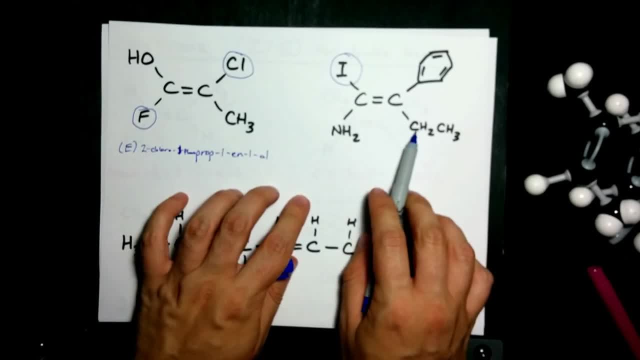 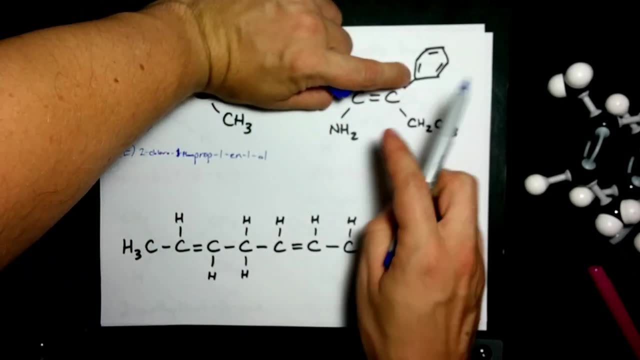 This carbon is connected to a fluorine. This carbon is connected to a fluorine. This carbon is connected to a fluorine. This carbon is connected to a carbon and a carbon. Those are the same, so we need to go one step farther. 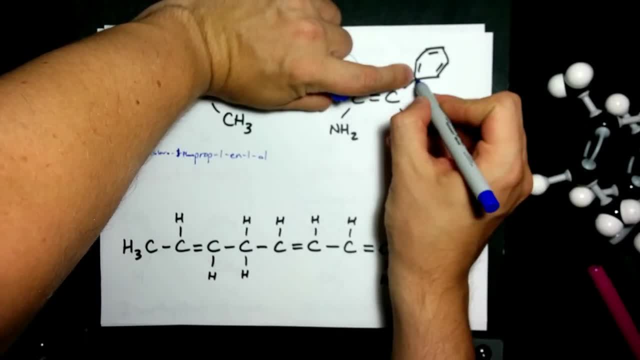 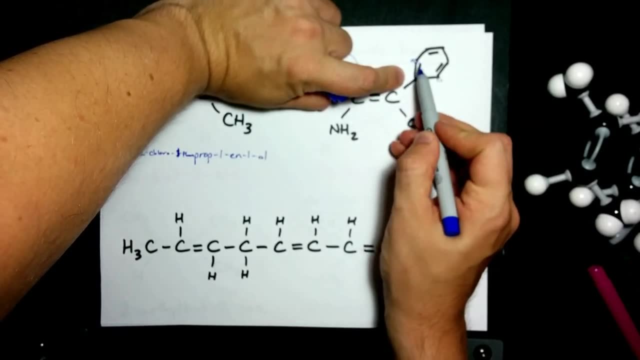 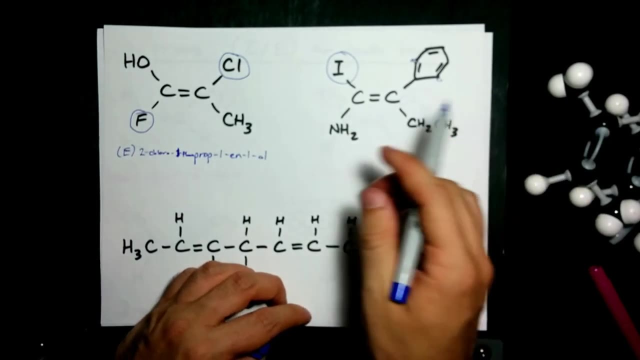 This is another carbon and two hydrogens. This carbon here is connected to one, two, three other carbons. Notice I'm double counting this one because it was double bonded. In any case, those extra three carbons. at the second bond, away from the central carbon, beats out the ethyl group. 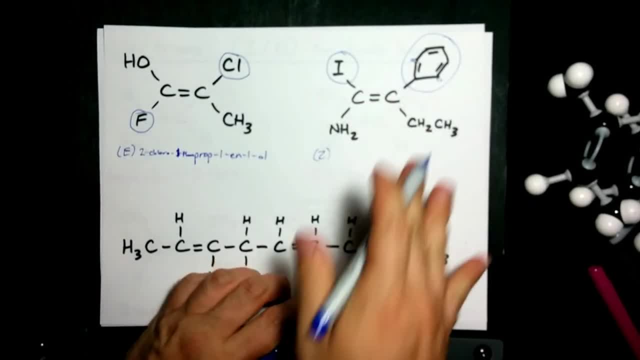 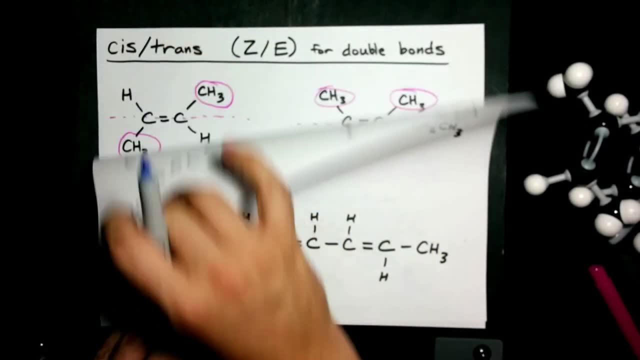 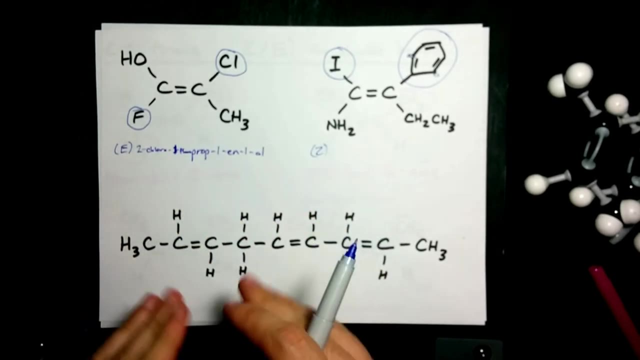 These are on the same side, so we call it Z And I am certainly not naming this. And finally, you might wonder why we had to create E and Z if cis and trans was working fine for us. Well, cis and trans gets really bulky, and I don't even know how to do it if you have more than one double bond. 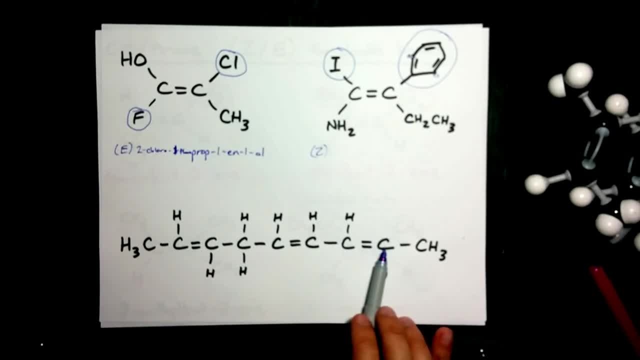 Here we have one, two, three, four, five, six, seven, eight, nine carbons in a row. That makes it a non, And the double bonds, I think starting from this side, gives us the lowest numbers. One, two, three, four, five, six, seven. 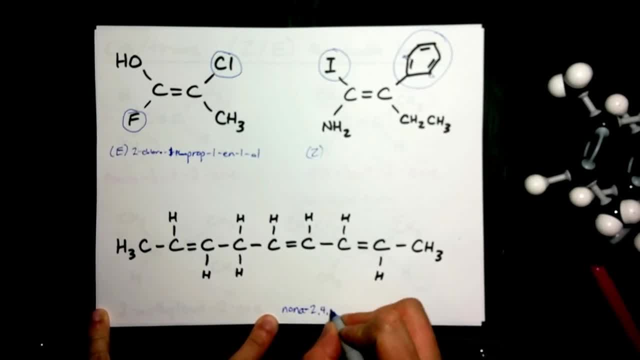 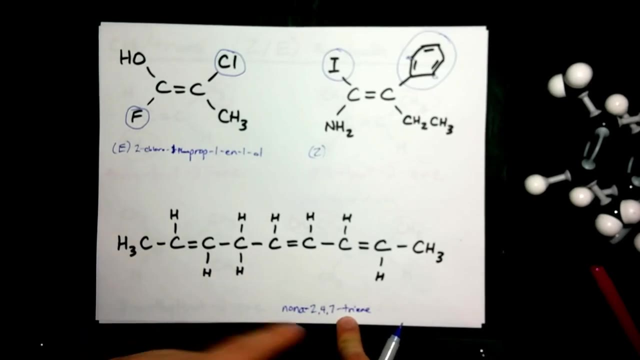 Nona, two, four, seven, triene, Three double bonds starting at carbon two, four and seven, And it's a nine carbon chain. I had to include this vowel because now the T is the next letter. It's a consonant. 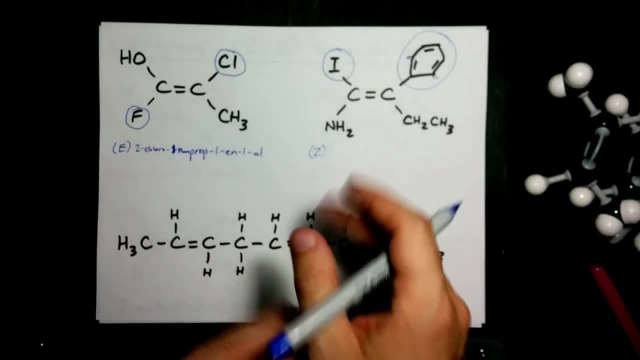 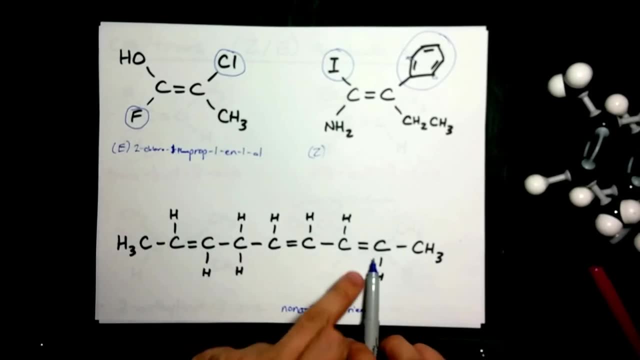 But what's really important to me Is whether or not each bond is cis or trans, And I can say that because I have hydrogens here. Let's start at carbon two. actually, Carbon two is here Now when you draw straight chain alkenes like this: 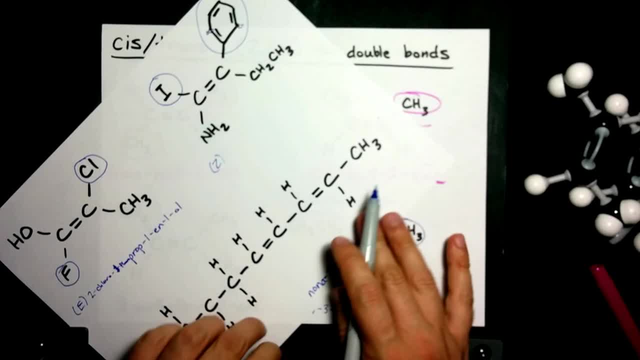 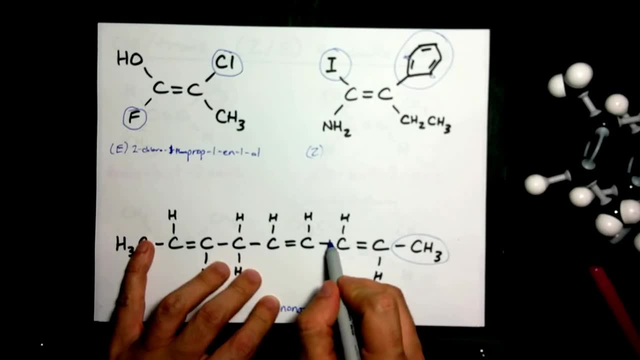 You got to remember these are actually 120 degree bond angles. All these angles are 120 degrees Because of the hybridization here, But that's CH3.. And this CH3 are on opposite sides of the double bond. That may not be easy to see for you. 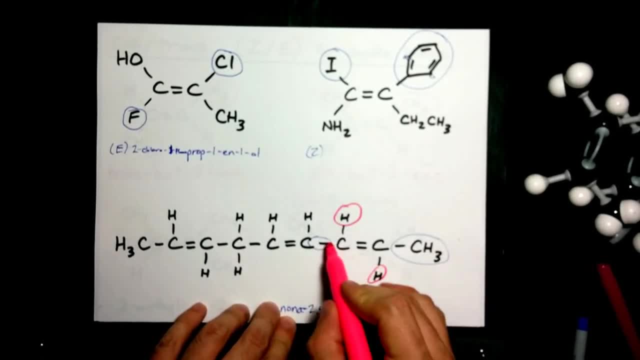 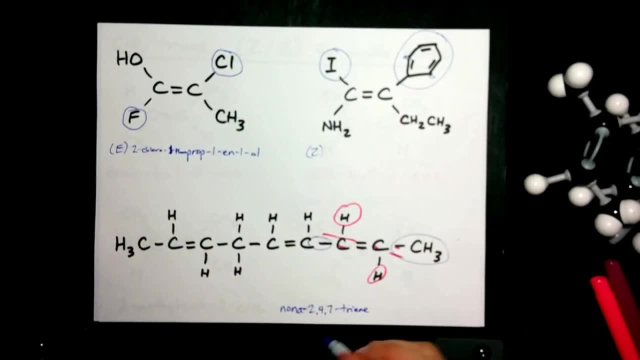 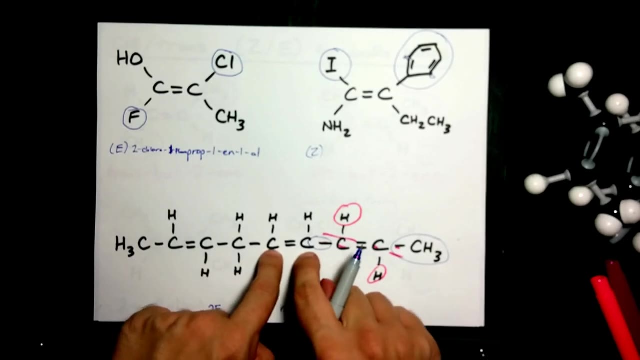 And so instead you can just consider the hydrogens. The hydrogens are clearly on opposite sides of the double bond. Great Opposite sides means trans, So we will say 2E. Okay, Here's another one. The two carbon linkages are both on the bottom half here. 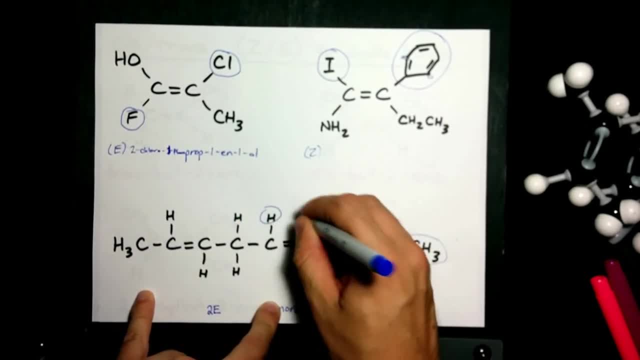 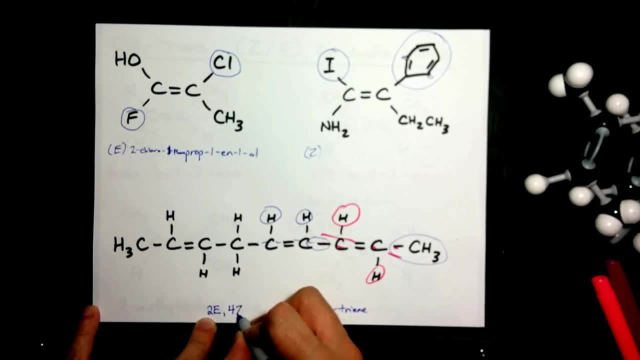 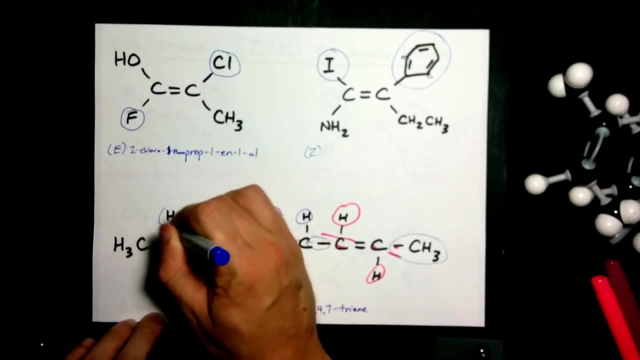 Or put another way, The two hydrogen linkages are both above the bond axis, So the double bond starting at carbon four is cis And finally, once you get to carbon seven. Hopefully you realize now that you can just compare where the hydrogens are. 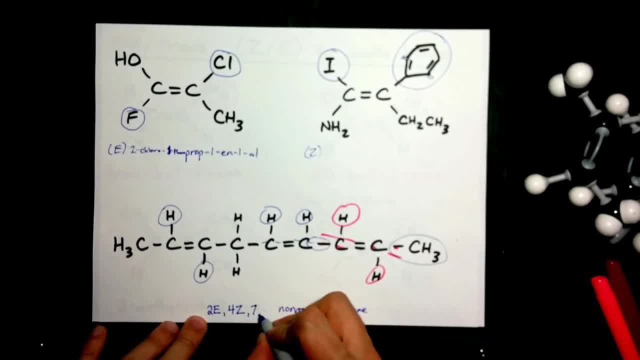 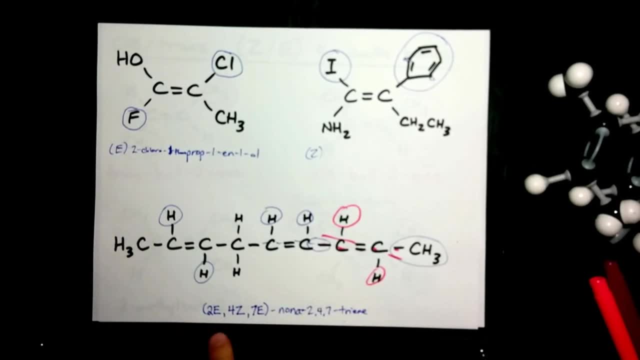 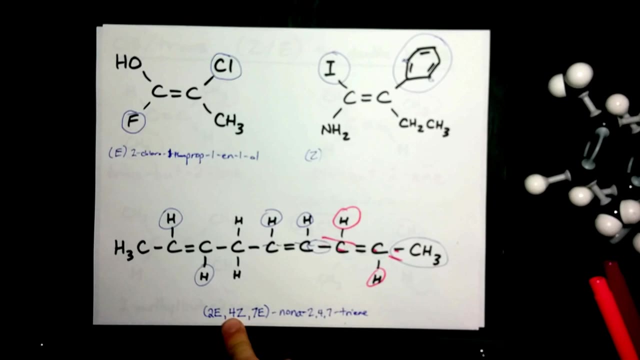 They're on the opposite sides, So that gives you seven trans as well. This is why it's so much easier with E and Z, Because you can just say: the double bond starting at carbon two is cis, The double bond starting at carbon four is Z. 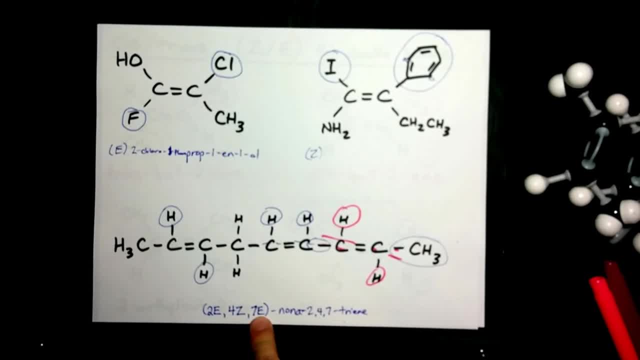 And the double bond starting at carbon seven is trans. I don't know if I got that right, But I did for the rest of the video And now you know. Good luck.